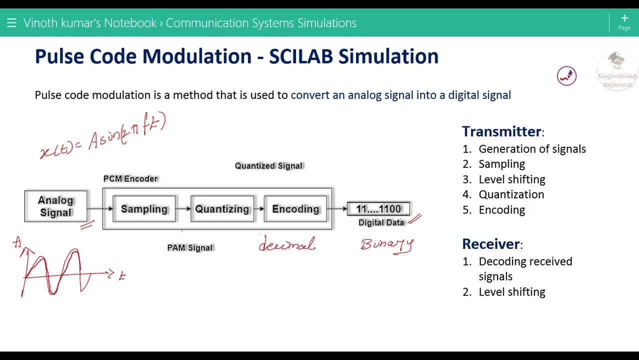 a sine 2 pi ft. The sinusoidal waveform is shown here and the sampler. here we follow the Nyquist sampling theorem, where the sampling frequency must be greater than or equal to twice the message frequency, and this is actually followed to sample the information signal and to avoid aliasing. 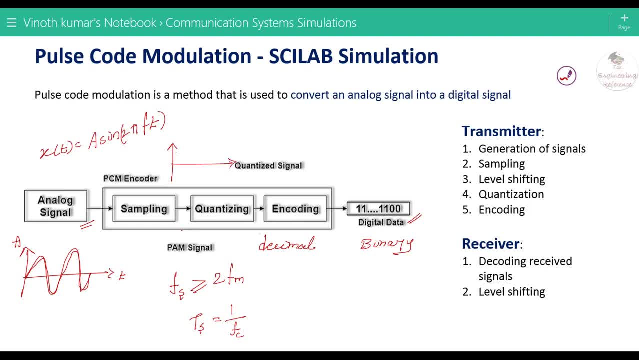 effect and all. So the sampled signal, the pulse amplitude modulated signal, is somehow like we will be having the continuous amplitude and discrete time signal and this multiple data, sampled data, are actually quantized by the quantizer where in Scilab program we will be. 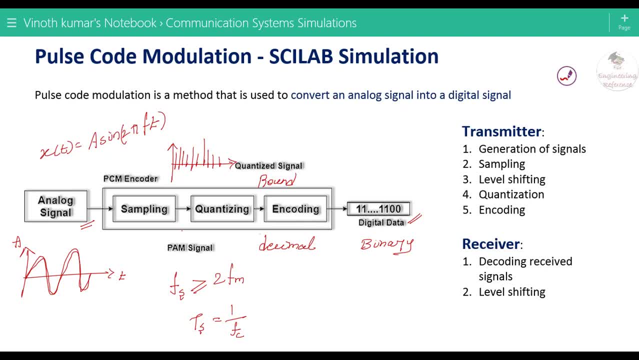 using round, the command round. So we are rounding the sampled value to the nearest decimal value. For example, if we have the sampled value as 1.76, it can be rounded to the nearest decimal as 2. or for these two â value, the sampled value is 1.12 and we round this value to the nearest decimal value. one. 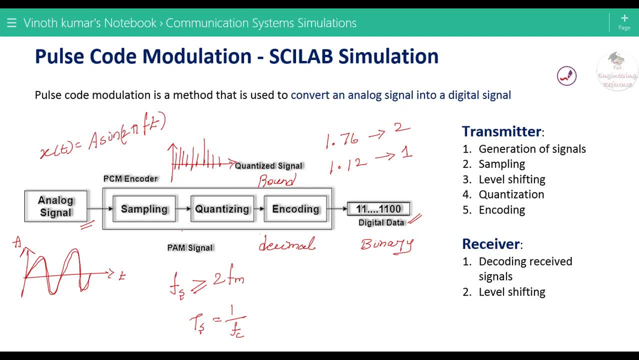 The corresponding binary values- zeros and ones equivalent to the decimal- is generated at the encoder, then it is transmitted over the digital channel And at the receiver side we first receive this binary data. so we need to convert this binary into decimal first. Then, from this binary to these two â value, we have one by one the value to be generated into the code and we turn them over to the digital channel, and at the receiver side we first receive this binary data. so we need to convert this binary into decimal first. 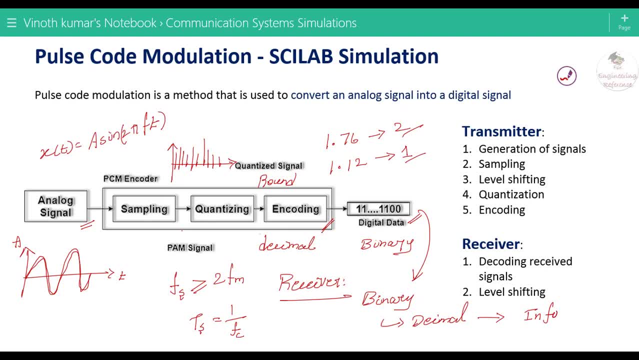 From this we will be extracting the actual information signal at the end. So these are the steps we are going to follow to write pulse code, modulation coding on Scilab platform. First we generate the signal. let us assume some variable: x is equal to a sin 2 pi ft. 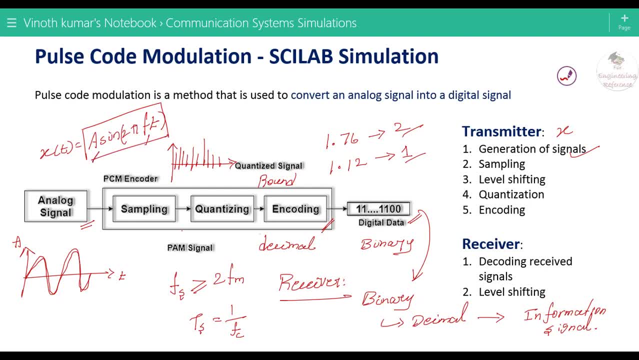 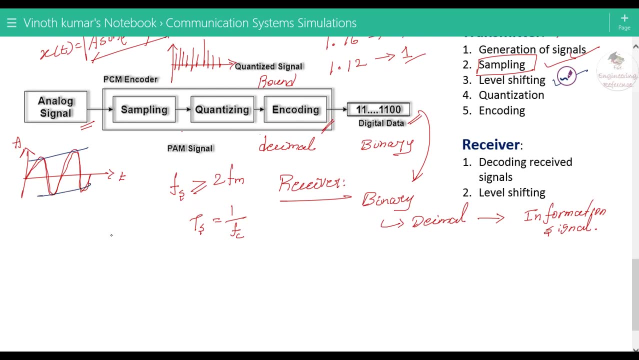 and we will be assigning some frequency value and the amplitude based on the Nyquist sampling theorem. we use sampling rate. So in level shifting the, actually the signal is having both the positive value and negative amplitude, positive amplitude and negative amplitude. here the signal is like this: having 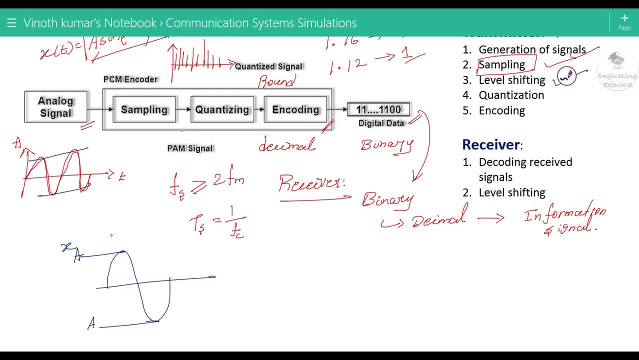 the positive amplitude and the negative amplitude. let us say, for example, adding a to these both amplitudes, We will be having in the positive cycle 2a and in the negative cycle minus a, plus a becomes 0. So this level shifting lets the process simple for quantization and encoding. 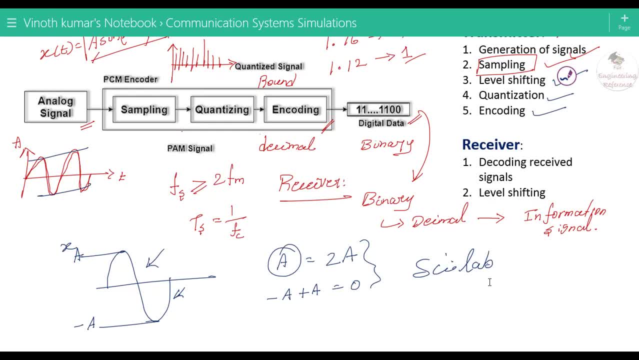 And in the Scilab platform. in order to quantize the signal, we can use the command round and to convert the decimal value to the binary value, we have the command round. Once again, I turn on the humanasion tool, Binary, and from Binary to decimal. 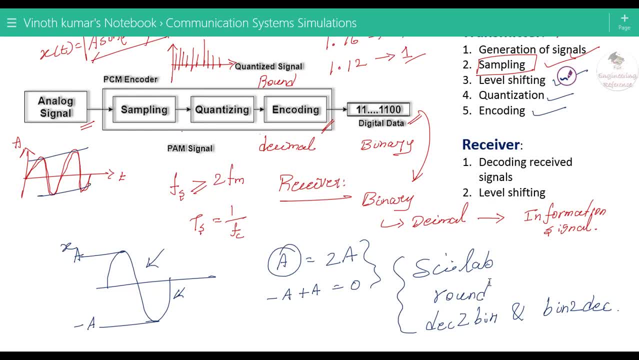 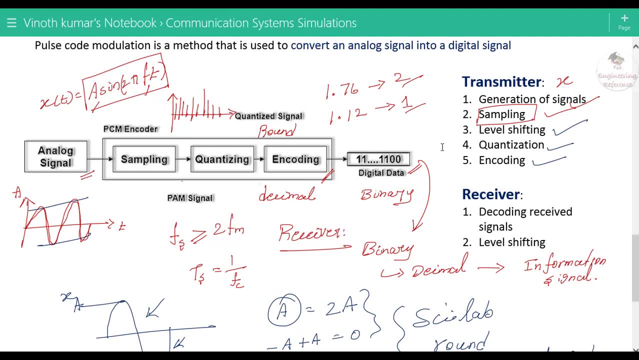 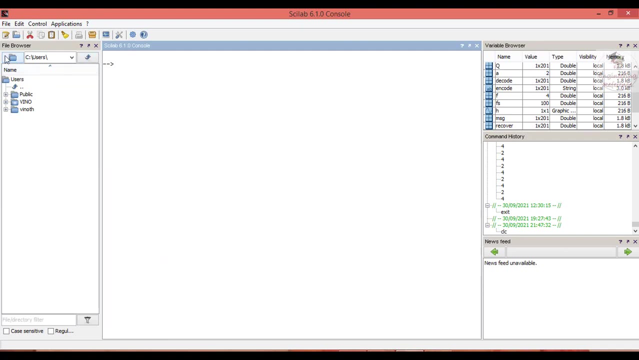 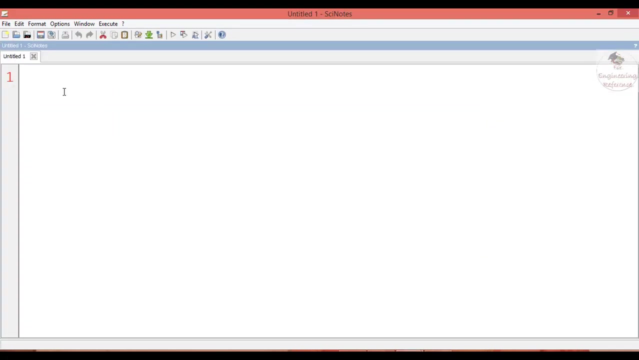 Let's see how to write the pulse code modulation for the transmitter receiver side, to transmit the signal at the receiver side. So I have already opened the Scilab software. I'm selecting both sides. now we may go to application and synodes. Here the synode page has opened. So basic commands. 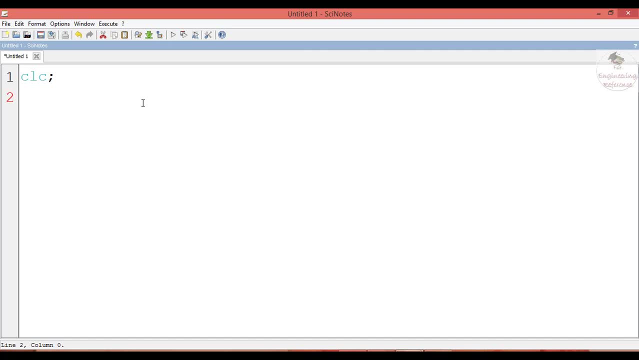 we use the CLC, the clear console. So this command closes the graphic figures and the progression bars and clear whatever the variable defined before are cleared here. So let us see the transmitter section. So double slash is used to write the command line. So in order. 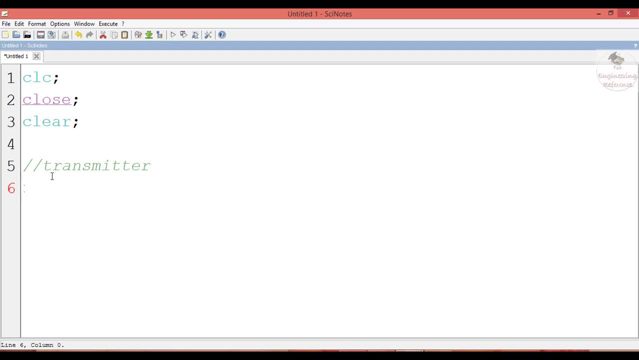 to generate the message signal. let me assume the frequency as 4 heads. We can use the higher range of frequencies, but having the minimum range of frequency will help you to view the waveform clearly. And the sampling frequency? yes, it should be greater than or equal to. 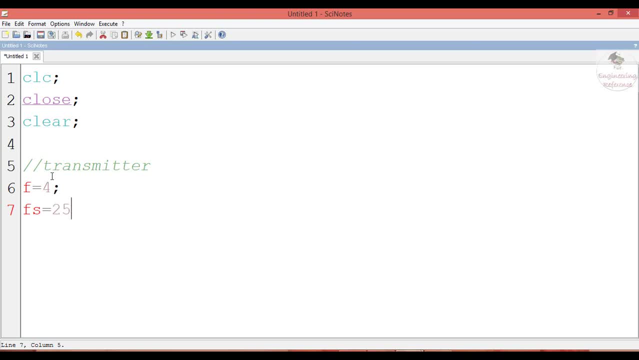 2 into fm. So let me write 25 into f. right, Some higher range, let us assume- and time period for how much time the signal is to be generated and, at the output graph, for how much time we are going to observe the waveform. So, starting from 0 and the incremental, it should be as: 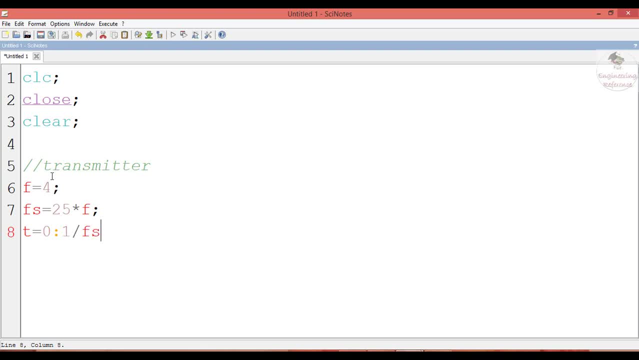 a sampling rate and it is given as 1 upon fs. the sampling frequency is to 2.. So the unstable product can also be written as 2 into f and as if the variable was different, from zero up to 2, starting from 0 to 2 and the increment as 1 upon fs. and for amplitude: 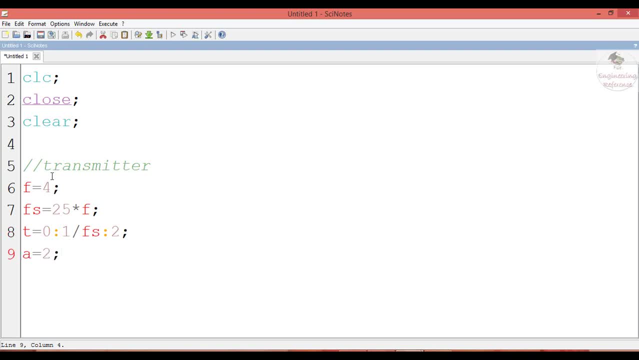 I take the variable A equal to 2.. I assign the amplitude to 2.. So the information signal, let me name it as message. By using the default, the function we can write, We can generate the sinusoidal waveform a sine 2 into pi. you know the amount of the amplitude, So It: is available to you for this, that is, the 104.125 Fs. a open amplitude is data very different than two sine 2 and pi 4.. So in order to determine the amplitude of this video, you just have to assume that the signal in the pattern of a positive expression or amount of the amplitude 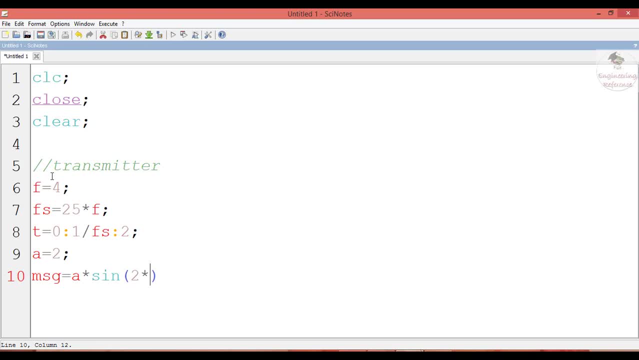 goes up to a large any Yexian which will be given. So eventually we take the importance of the terms Pi. you know the Pi value in CYLA platform is to be given as percentage Pi. so 2 Pi f into t. So this is the message signal, right? Let me put it in the message signal right. 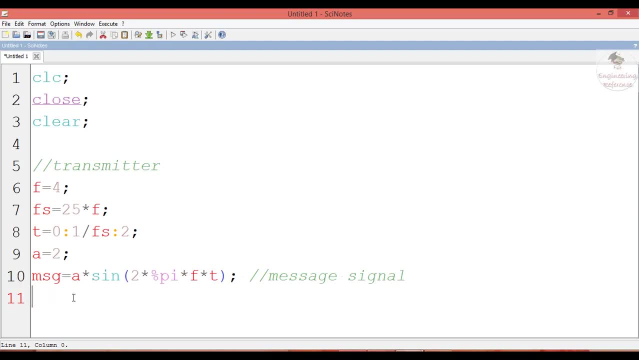 In order to plot all the graphs of this pulse code modulation program, I take the command subplot where I have. I'm going to have a three graph in a window, the first column and first picture. I'm going to plot this message signal. So the command to plot the 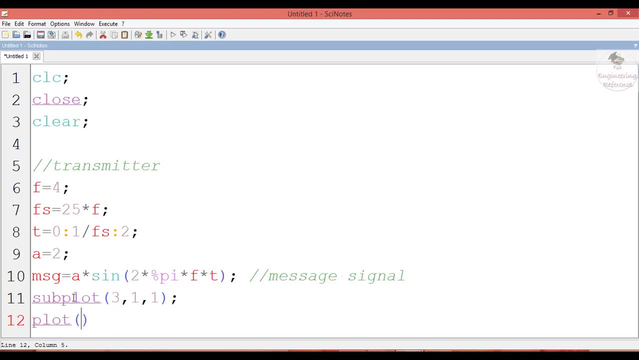 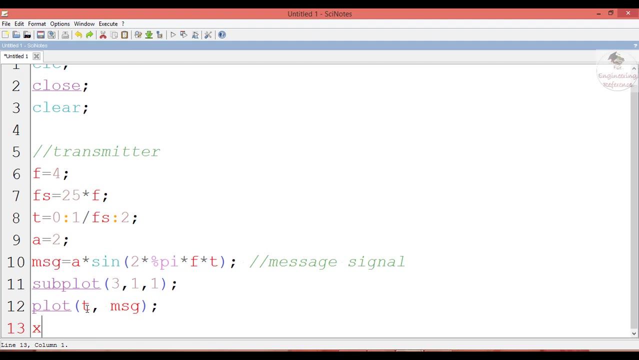 signal is plot of for the way time period, So here time we assigned as t, So for t comma, the message signal signal to be plotted is the message signal. And yes, we can use the name, the x axis and the y axis using x label and y label. So inside the code let me give: 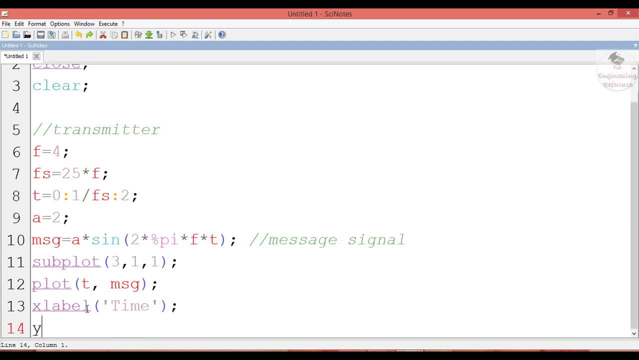 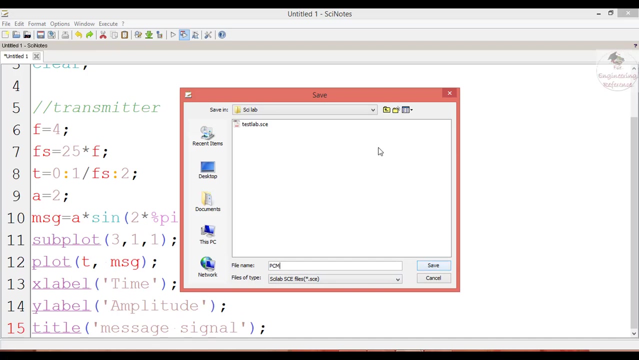 it as time and y label This we can. it is amplitude. Then the title of the graph can be given as title of message signal Right? Yes, So let us save this and execute. So, PCM. it is saved as dot se File, Right. 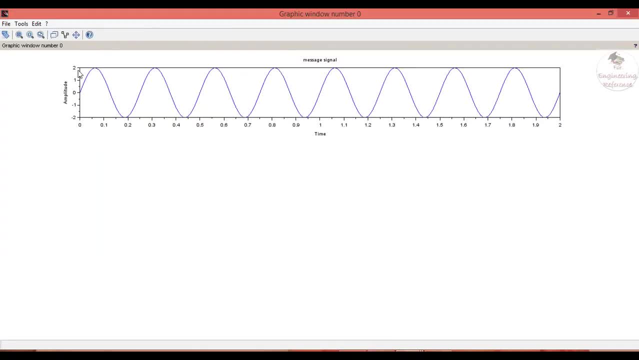 Yeah, So this, look at the amplitude. it is plus two and minus two, So two into sine two, pi ft, f is the amplitude, therefore t, So t, comma t, what two. this is value, you know, yes, Yes, yes, Enjoying this video, Alles bis zum Euchomesen. 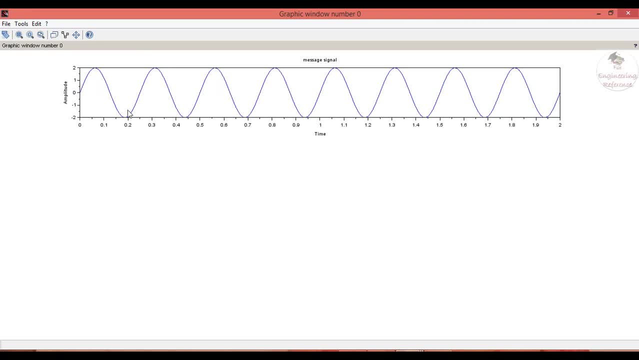 frequency f we assigned as 4, so 1 upon 4 is 0.25. so that is why for single cycle we have the time period 0.25. here and in x axis we are having the range starting from 0 and ending at 2, as 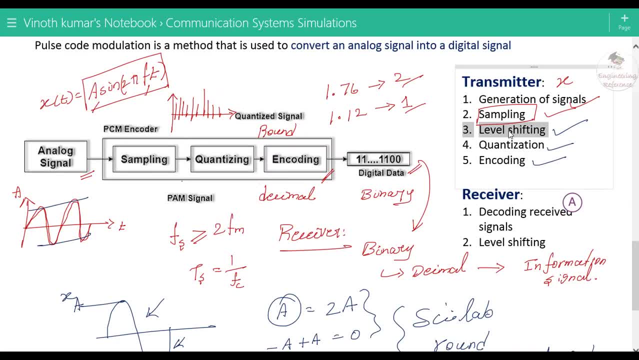 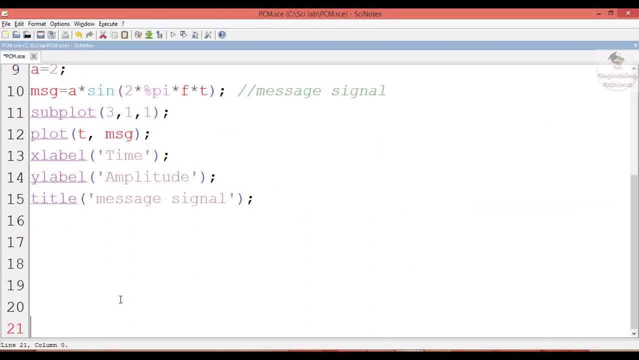 the time we defined. So next we are going to do the level shifting and quantization and encoding at the transmitter of false code modulation. For the level shifting I use the variable x is equal to the information signal message plus the value we assigned for the amplitude I use. 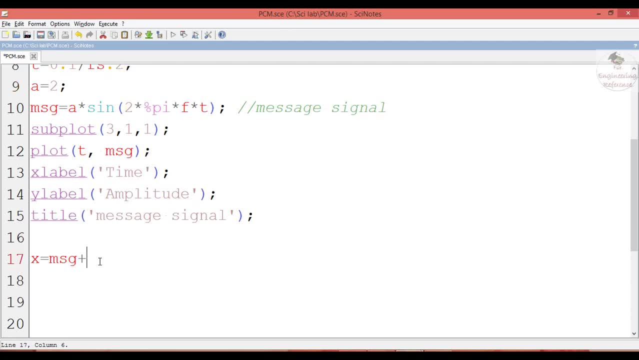 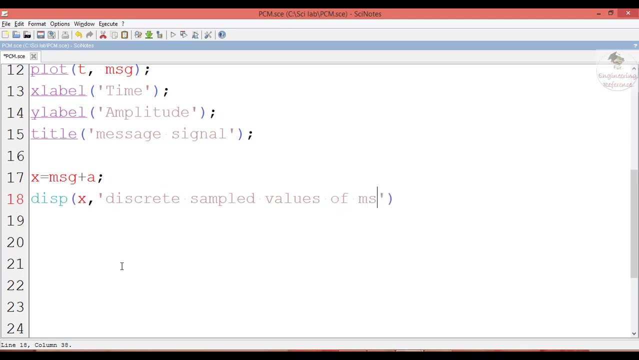 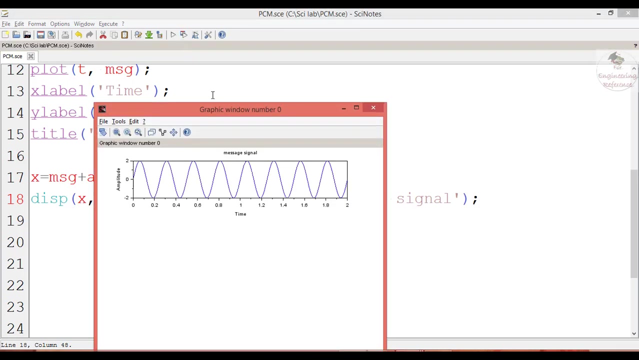 the same value to shift the signal level right, a. and if we want to display this value we can use the display command disp, ti, sp, sp, r. so this x is nothing but discrete sampled values of the message signal right. so let's check again. let us check this in the command the discrete values. so these are the discrete. 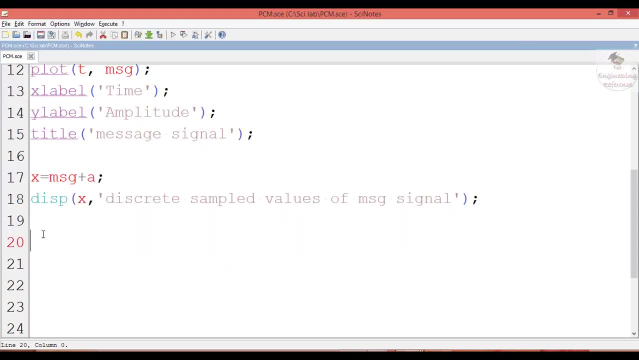 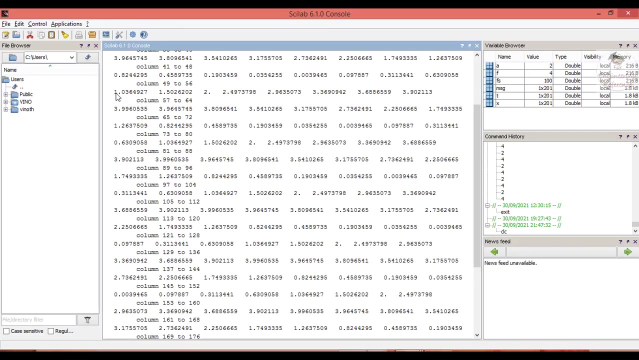 values of the message signal. right after the level shifting. we do quantization. so for quantization I use the variable capital. q is equal to the command round off. so here the discrete sampled values of the message signal as 1.03, 3.99, 1.26. so we are going to round these values into to. 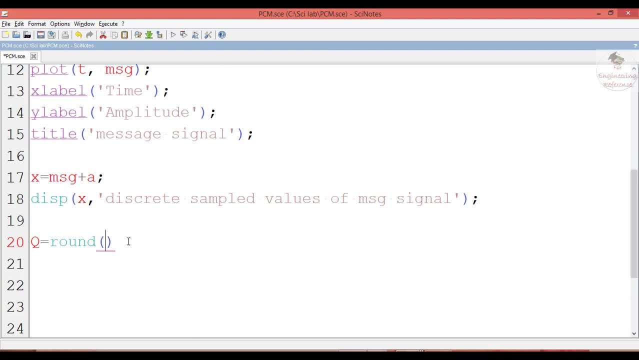 the nearest decimal value, right? so the discrete sample signals are x. so we can verify this also by displaying, ah, ah, the values of q, comma. So this is actually nothing but quantization of quantization of sampled signals, right? So next we are going to have the binary equivalent of the decibel number, so encoding process. so for that we, I use the variable. 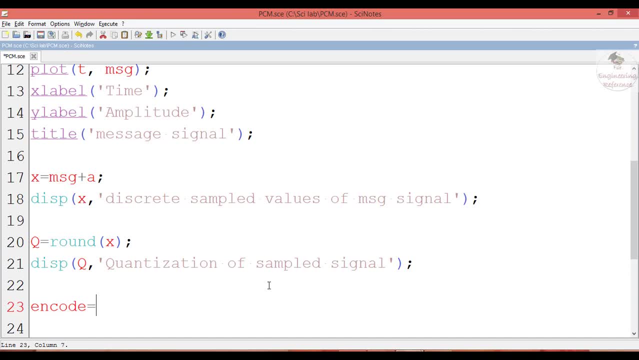 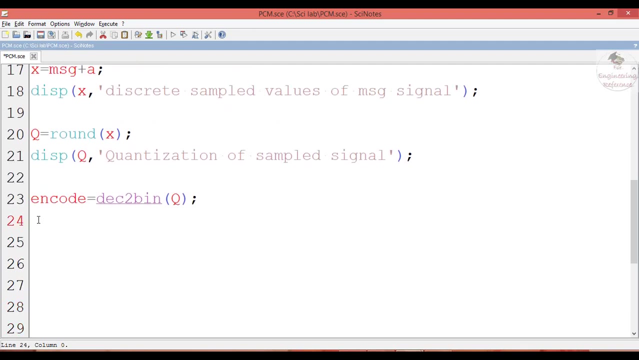 ah, n code is equal to. in order to convert the decimal to binary, we use the command decimal dec to bin of the quantized signal q, right, so let us verify this one also: display of n code. and this is actually digital signal. let's say this is the digital. 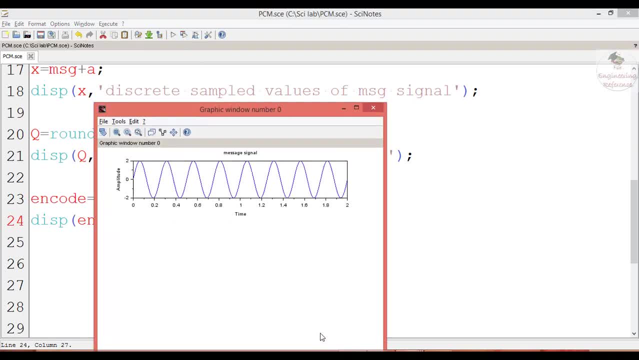 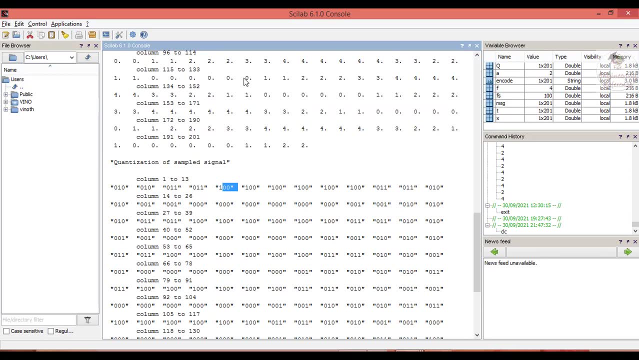 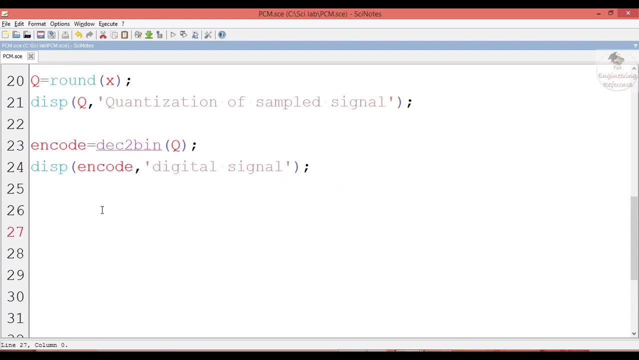 signal. here we are getting the binary equivalent of the above decimal value. so this is what performed at the transmitter side, then at the receiver side. receiver side, we need to extract, we need to receive the binary signal, and at the receiver side we do receive this binary data. and here to 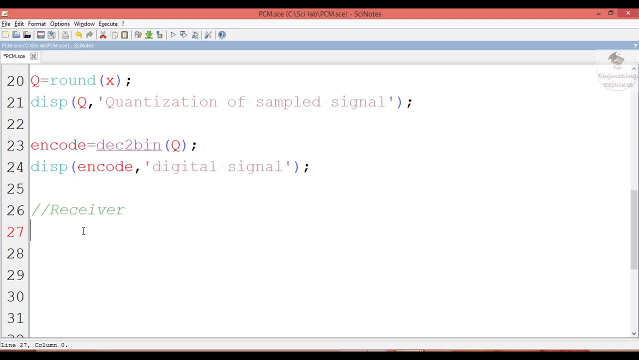 convert the binary into decimal. then from the decimal value we extract the information signal. the first process at the receiver side is decoding, so i use the variable decode. so for that binary, 2 decimal of the information received here is encode. right, yes, yeah, this will have the decimal value and we did the level shifting. right now i am going to 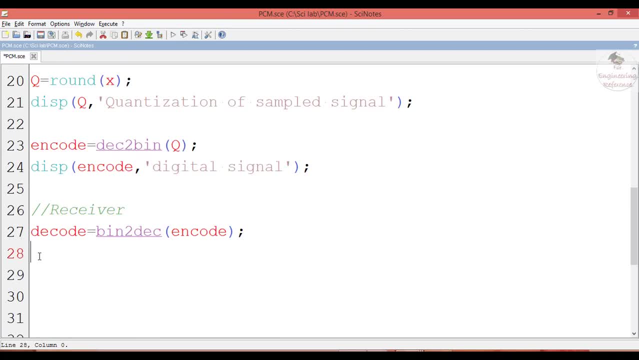 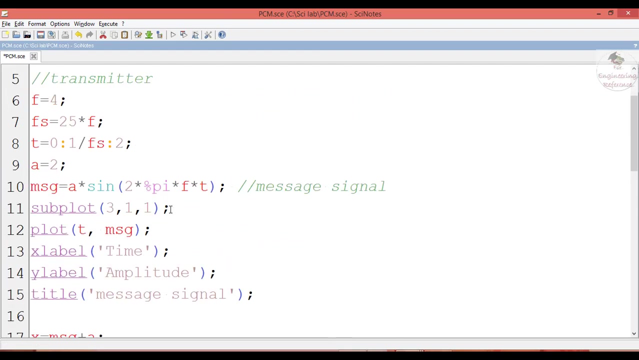 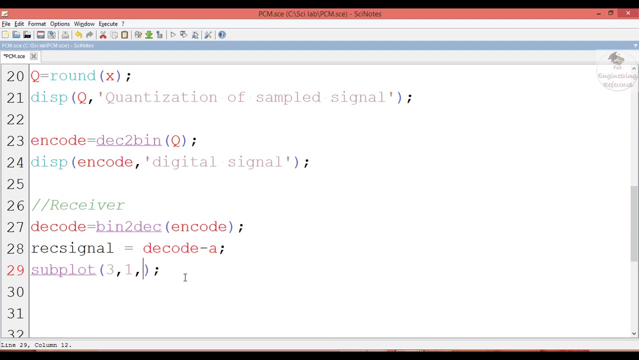 subtract this decoded signal by minus a, so recovered signal, REC signal, let me say: recovered signal is equal to, so here decode, minus a right recovered signal. So let us check this plot, let us check this waveform, recovered signal, waveform. So I am going to use the same subplot command here and in the window the second picture. 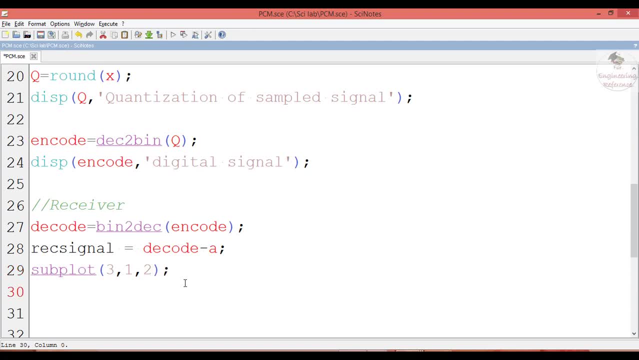 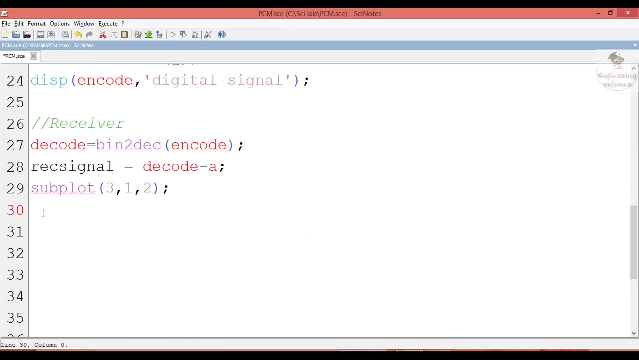 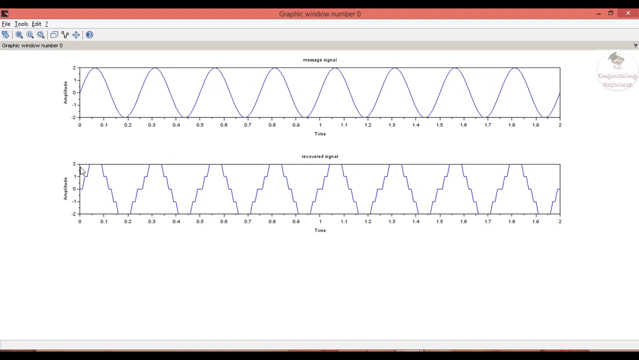 I am going to view this recovered signal right, So remaining, I copy and paste the same commands. so plot of here: T comma- REC SIGNA- recovered signal. So this is recovered signal. so save and execute. yeah, So this is the recovered signal. Look at the scale of y axis. we have the maximum value, 2, and minimum value minus 2 in the graph. 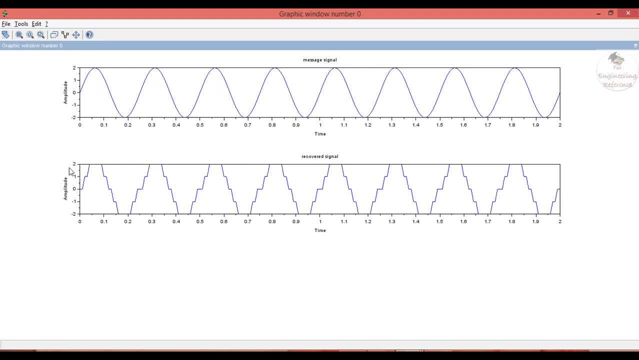 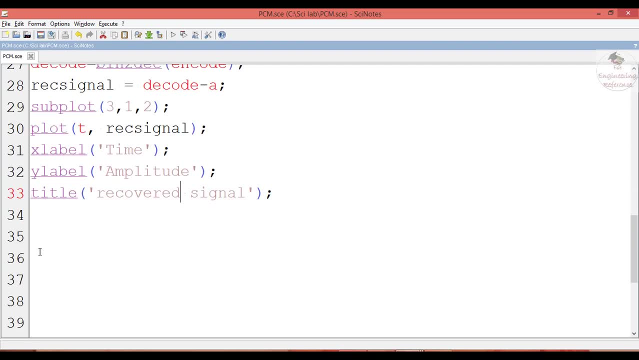 and in order to view this waveform clearly on the graph sheet, we can change the x- y axis parameter as like. go to. now let us use, for example: h is equal to g, c, a, which is, which means get current axis. it holds the current axis And in this the data bounds x and y axis parameters. right data command used to arrange the scales. 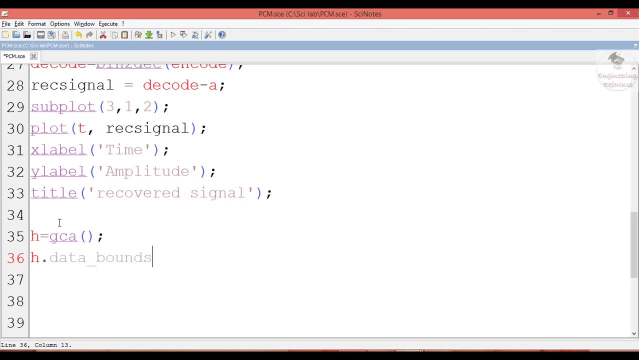 h dot data bounds equal to what should be the minimum and maximum value in the x and y axis. Let me give it as 0 comma Minus 3.. Okay, and 2 comma 3.. Let us have the comparison of the recovered signal and the information. 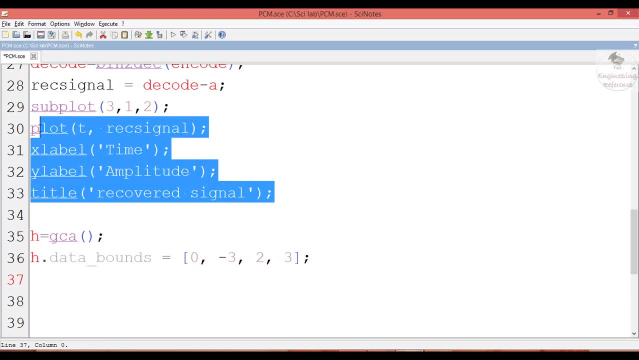 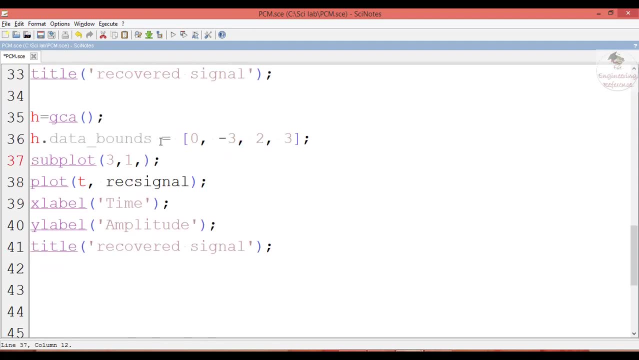 signal. So for that again let me take these commands. So subplot of the third picture right. third picture: here first let me plot the message signal, then the recovered signal right on the same plot for the comparison. So here recovered signal versus the message. 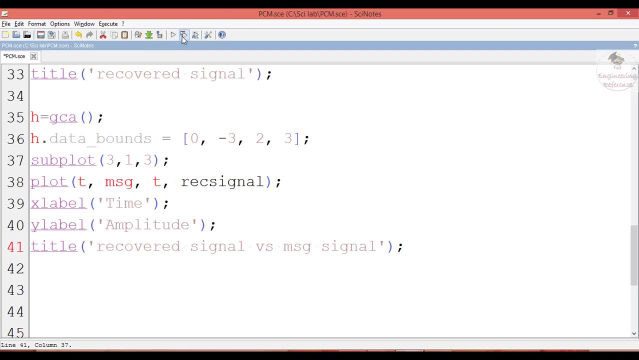 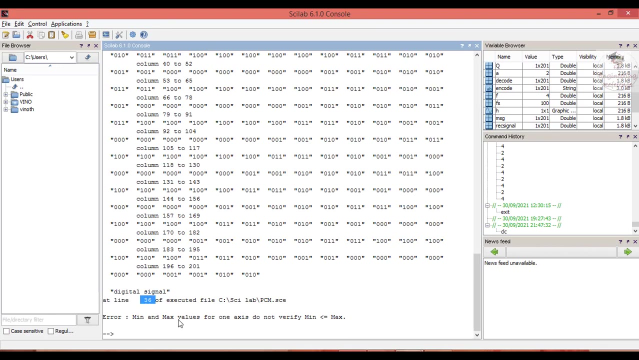 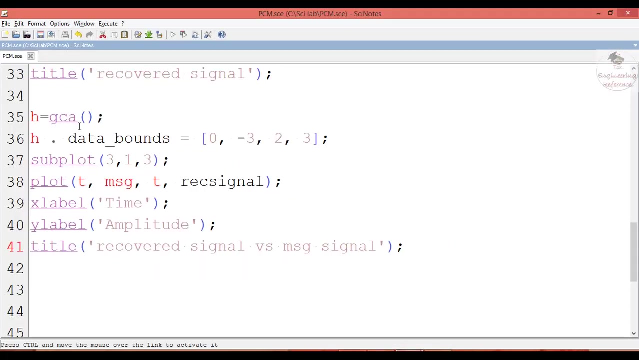 signal right, yes, now save and execute. So the third plot is not displayed here. so there is an error. the error is actually at line 36. the minimum and maximum values for one axis do not vary. minimum distance are equal to zero, the maximum, so at line 36 we are having this error. so 36, so it is x axis 0 to 2, y axis minus 3: 2. 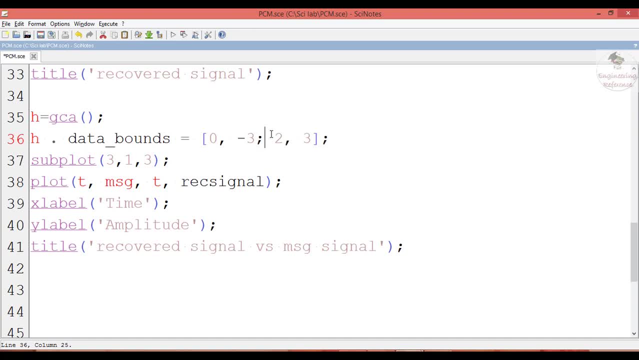 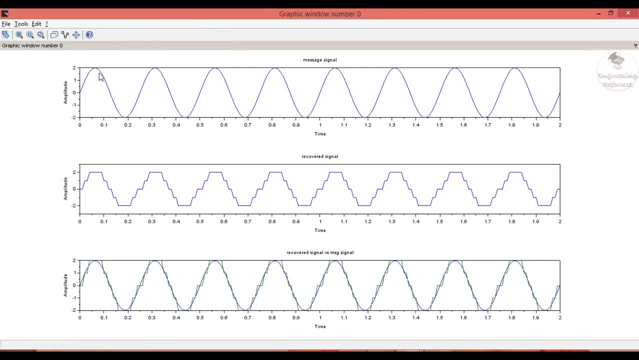 okay, here, instead of colon, we need to give semicolon right. so save and execute. yes, now we are getting the plot. so the first one is the message signal. second one is the recovered signal, so you can check that y axis starting from minus 3 to plus 3, and the recovered signal and the